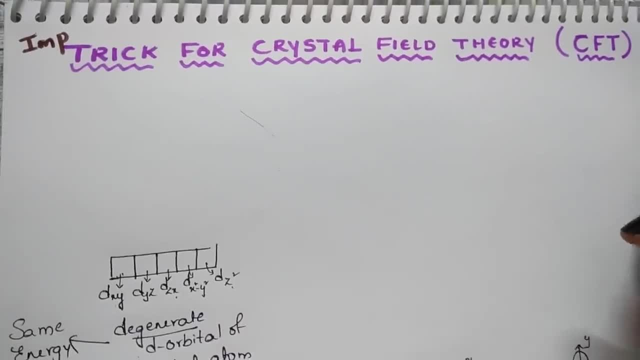 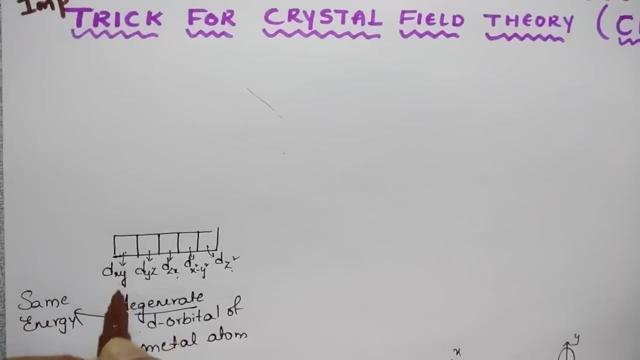 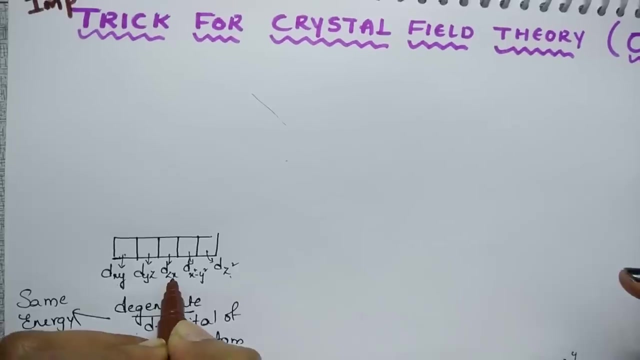 as well as tetrahedral complexes. Let us start our session. Metal consists of d-orbitals. These d-orbitals are: 5 d-orbitals will be present. One is dxy, dyz, dzx, dx, square minus. 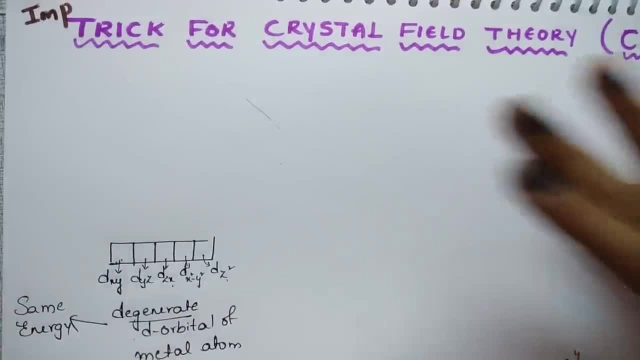 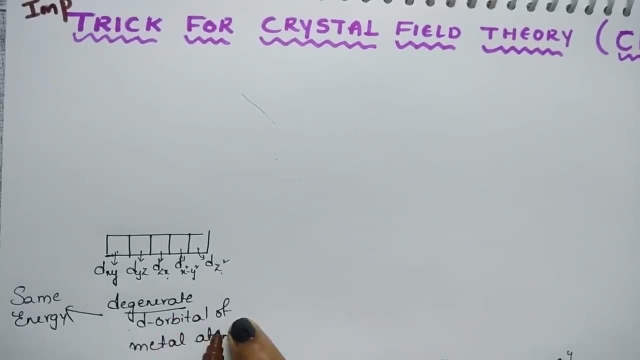 y square, dz square. These are the 5 d-orbitals. These 5 d-orbitals which are present in the metal, we call it as degenerate d-orbitals. The reason is these 5 d-orbitals are having 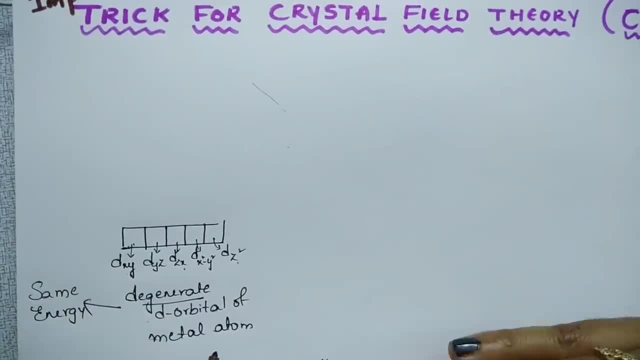 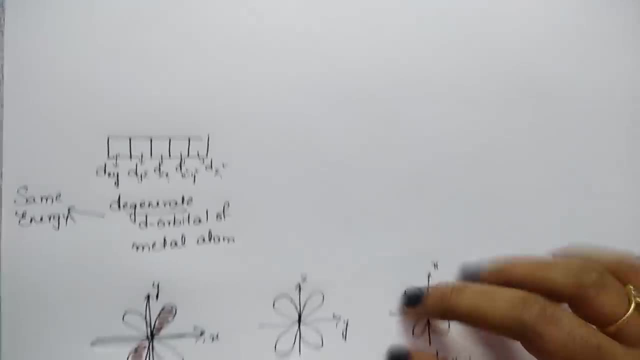 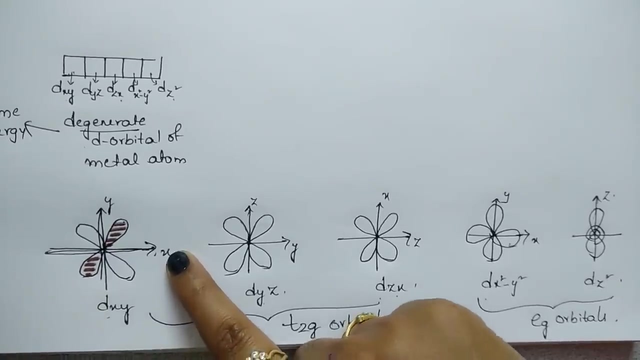 the same energy. That's why we call it as degenerate d-orbitals. Electron can enter into any of the d-orbital And these are the structures of these d-orbitals. This is the x-axis and this is y. Let us assume that, And if the lobes of the d-orbital are? 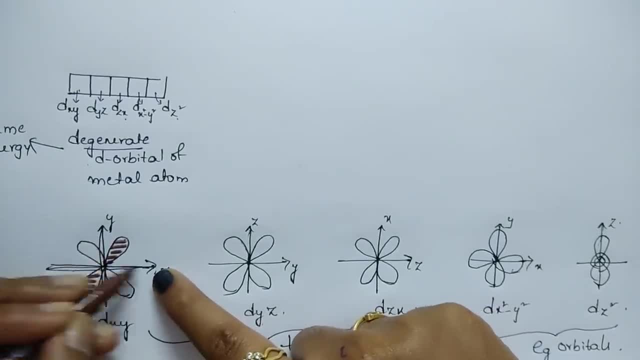 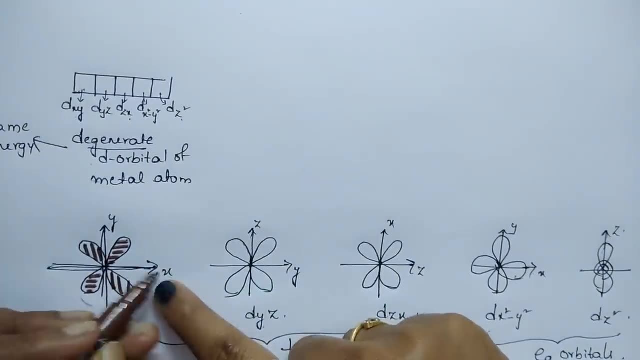 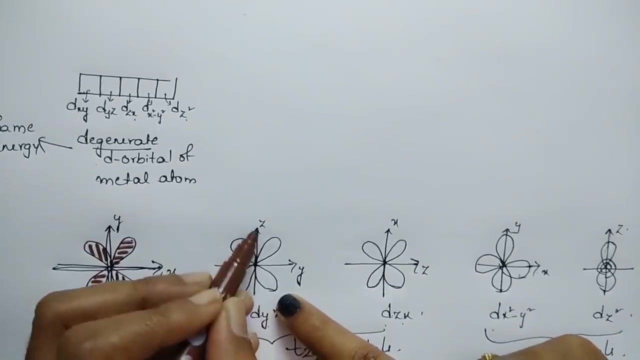 present between the axis. This is the axis And between the axis, if these lobes are present, we call it as dxy. And here also, if you see, these lobes are present between the axis. This is the axis and this is one more axis, And the lobes are present between the axis. 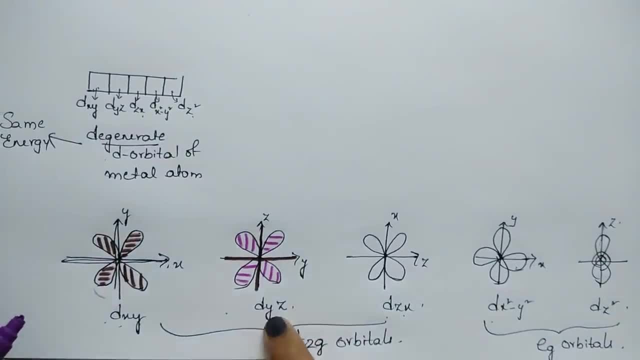 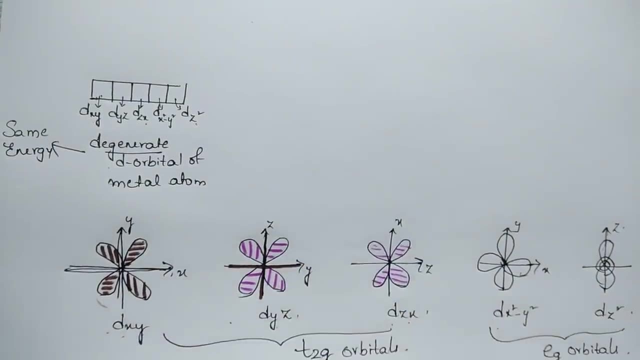 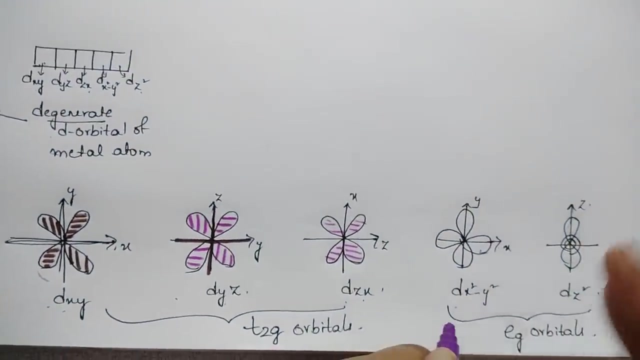 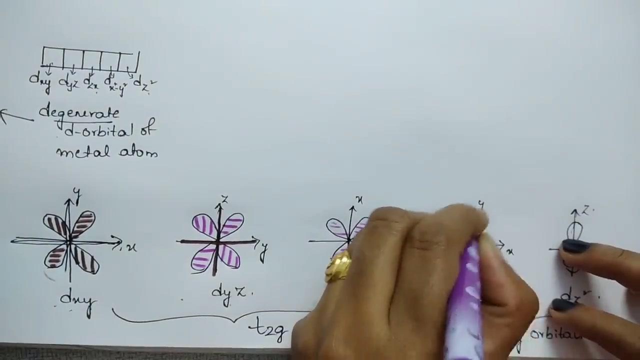 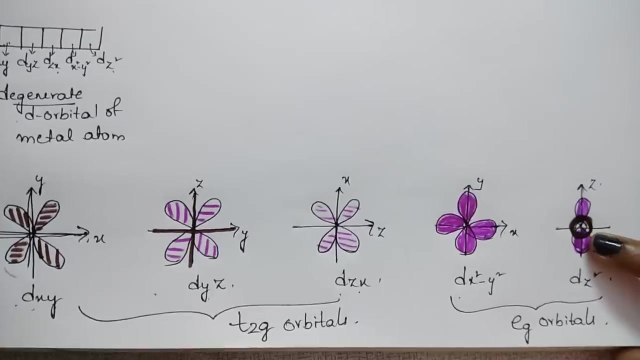 We call it as dxy. Sorry, this is dyz And this is dzx Here. in this case, dx square minus y square and dz square. Students, if you observe, the lobes are present along the axis Here: dx square minus y square and dz square. 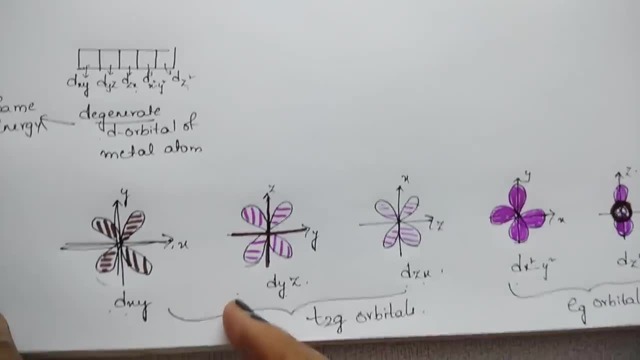 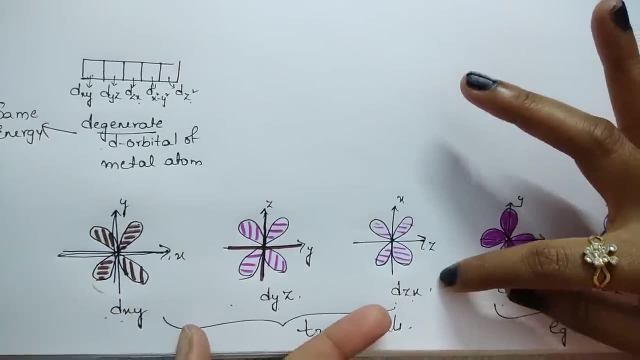 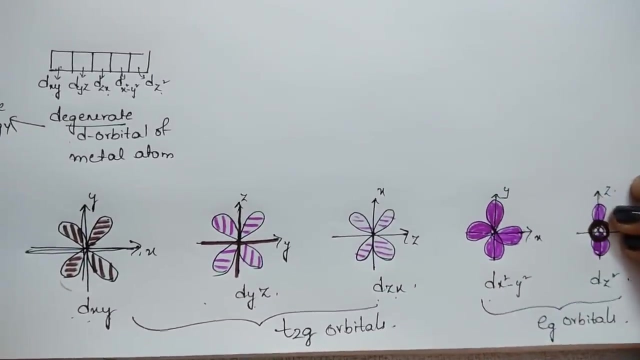 the lobes are present along the axis. The case where the lobes are present between the axis For these three d-orbitals- they are named as, according to the spectroscopy, t2g-orbitals- And the case where the lobes of the d-orbitals are present along the axis. 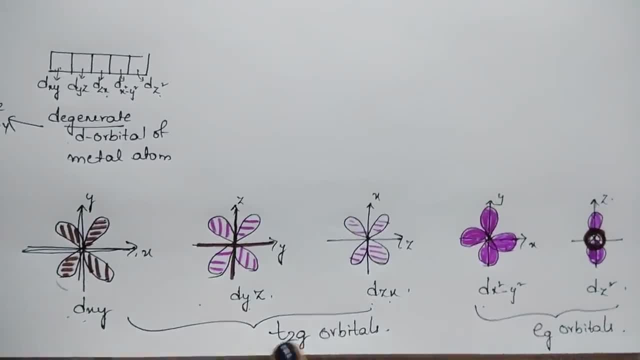 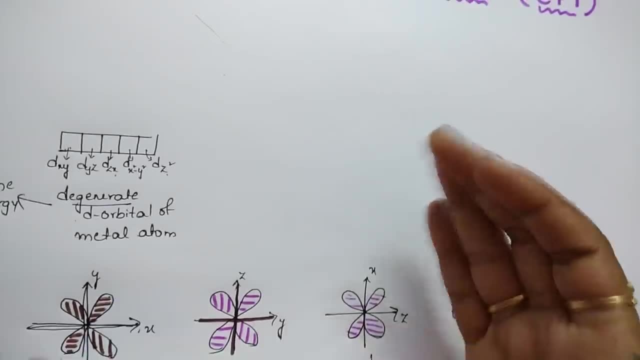 named as eg-orbitals. How I am pronouncing t2g Here. eg-orbitals Means d-orbitals. consist of two sets Again. one is t2g-set, another one is called as eg-set. 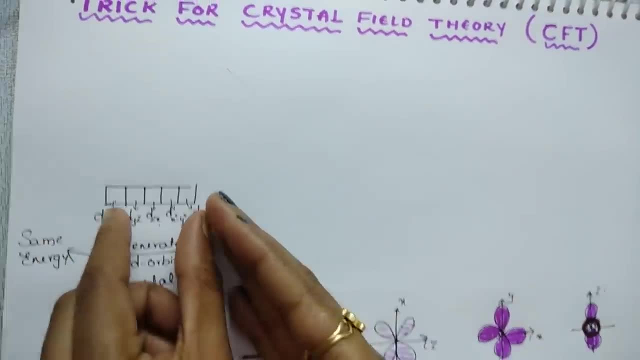 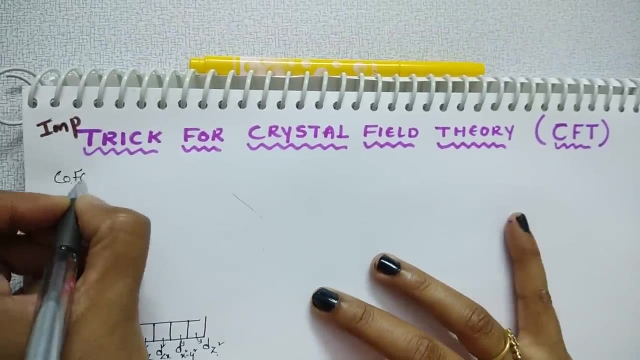 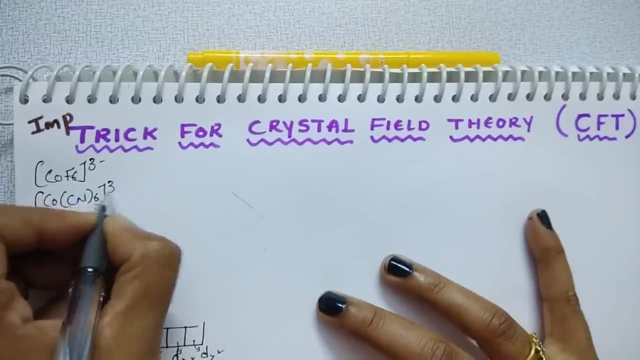 d-orbitals. all the d-orbitals are having the same energy. Up to here, clear students. Now what happens is if you see a complexes like COF6-3 or COCN6-3, this case of I gave. 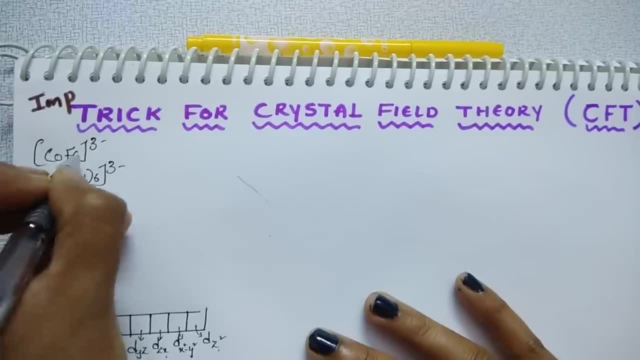 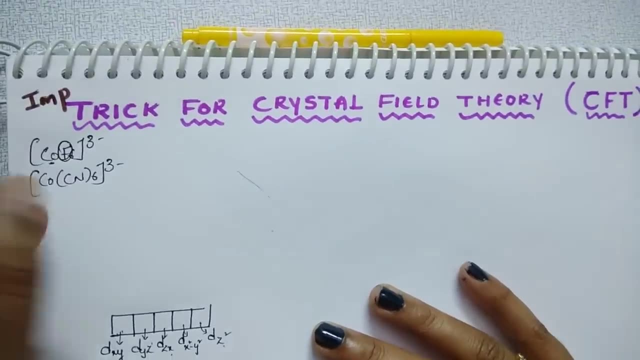 two examples, In this case of. in this case, what happens is: this is a metal. We discussed about the metal which consists of d-orbitals. Right Now, this fluoride ion, or cyanide ion, it approaches the metal to form this: 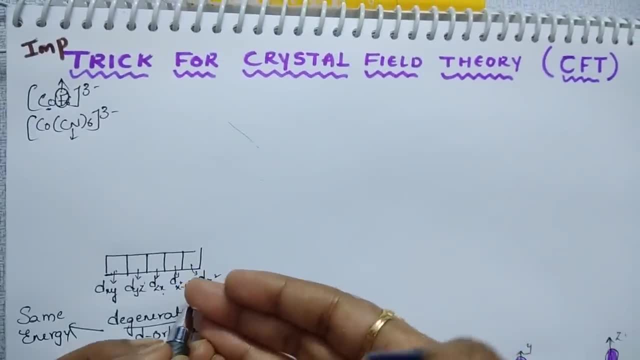 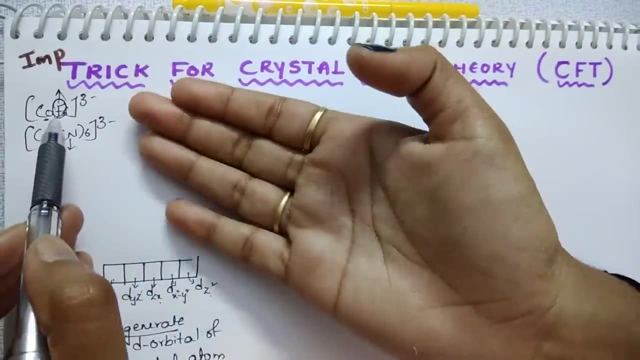 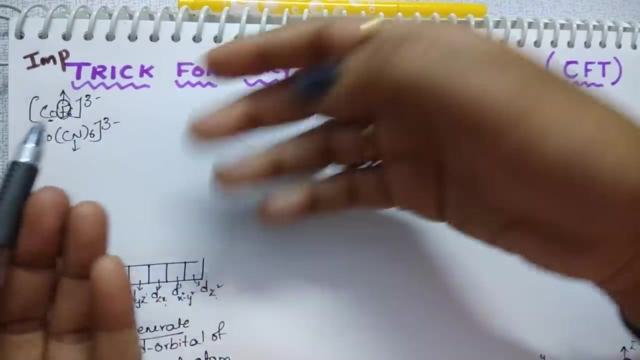 complex. Initially, this is the metal which consists of d-orbital, And this ligand approaches the metal to form the complex. Then what happens? Metals consists of electrons, d-orbitals, which consists of electrons, And these ligands also consists of lone pair of electrons. Whenever. 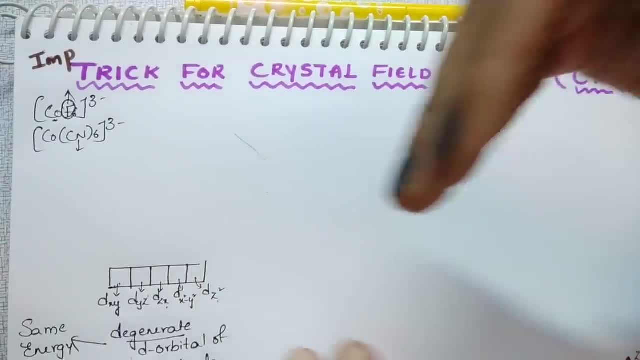 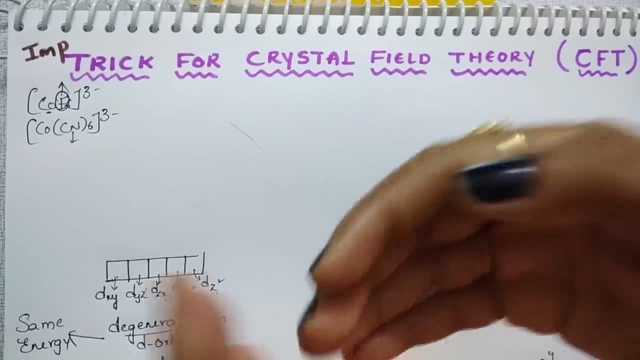 these ligands approaches the complex, they form a complex. So this is a complex, So this is a metal. There will be a repulsions between the ligands as well as these d-orbitals. Whenever there will be a repulsions, then these d-orbitals energy, it loss its degeneracy. 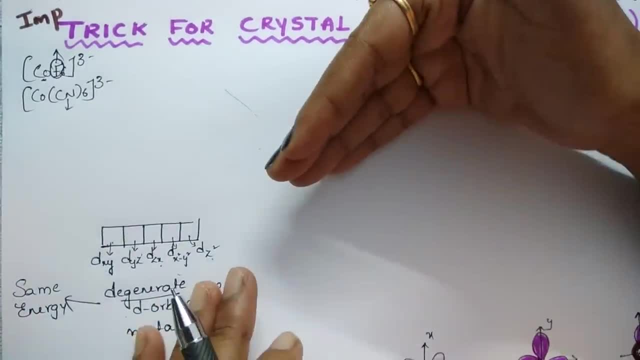 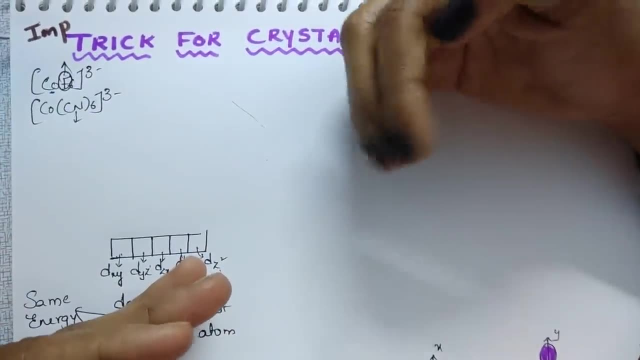 Why it loss its degeneracy? Because when ligand approaches, metal also consists of electrons and these ligands also consists of electrons and there will be a repulsions between these two. Then, whenever there is a repulsion, then it will be a repulsion. So this is a 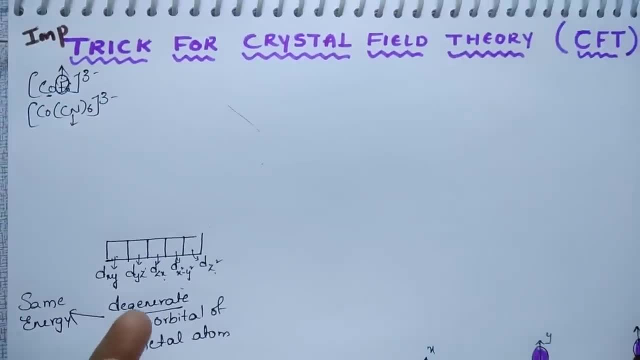 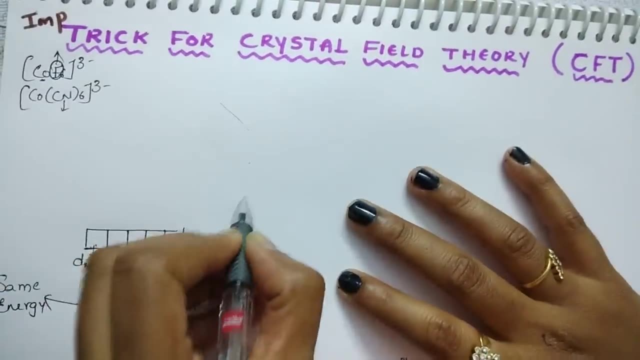 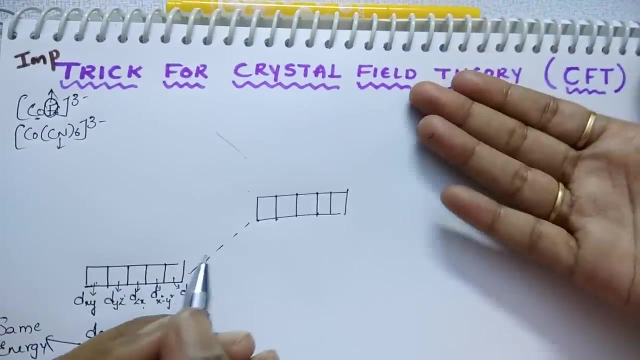 repulsion, The d-orbitals will be loss its degeneracy. When it loss its degeneracy, then what happens. See here: when ligand is approaching, the energy of the d-orbitals is not same. That is the meaning of loss its degeneracy, What it means: The energy of the d-orbitals. 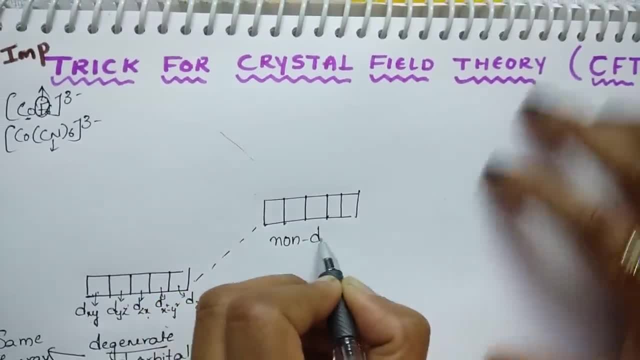 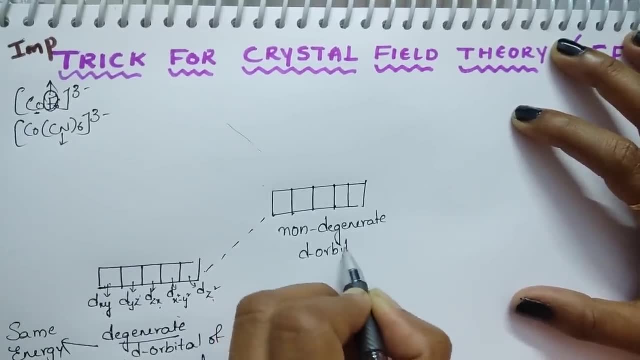 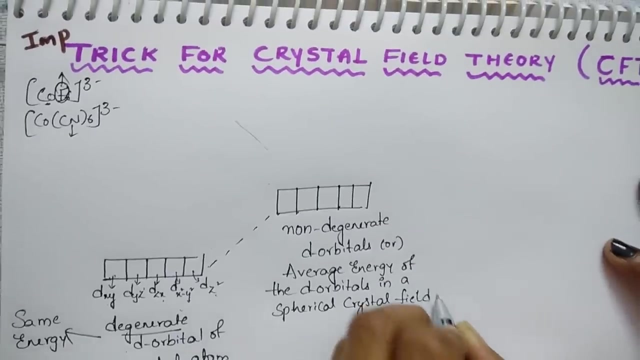 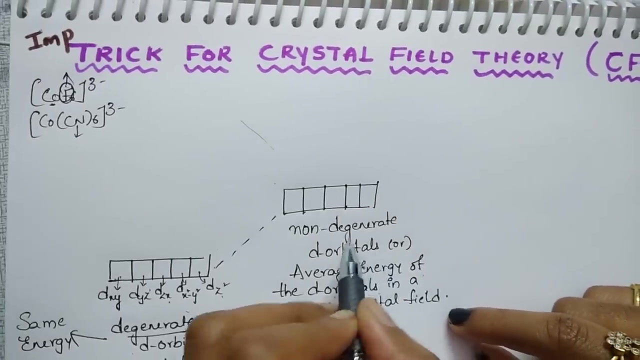 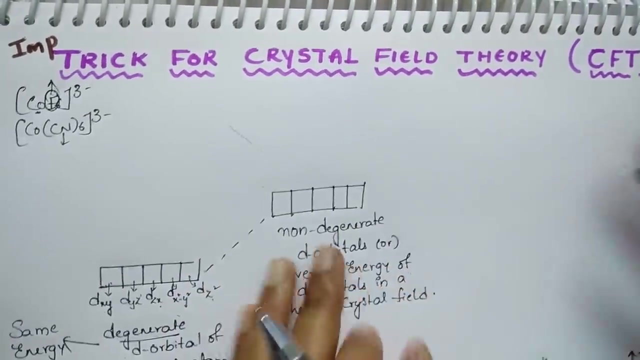 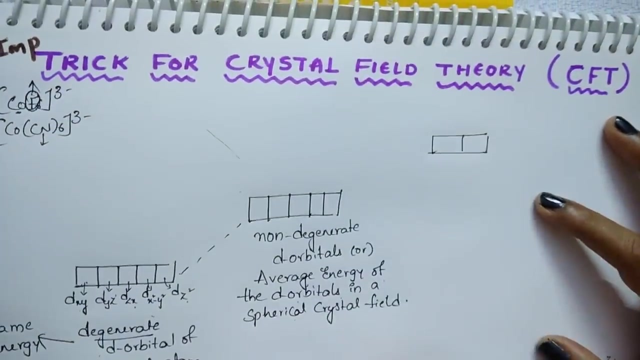 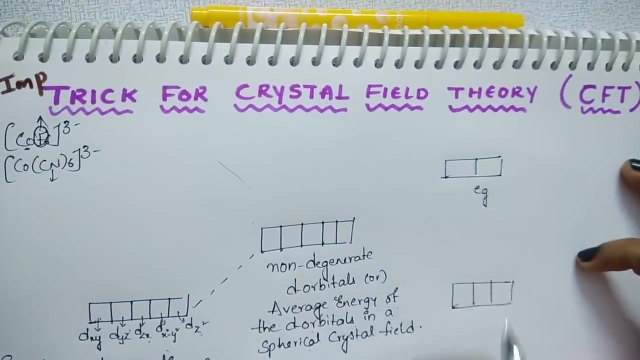 is not same. We call it as non-degenerate d orbitals, or average energy of the d orbital in a spherical crystal field. you can say: non degenerate d orbitals are average energy of d orbital. this, these non degenerate d orbital, get splits into two sets. one set we call it as EG set and other set we call it as T2G set. 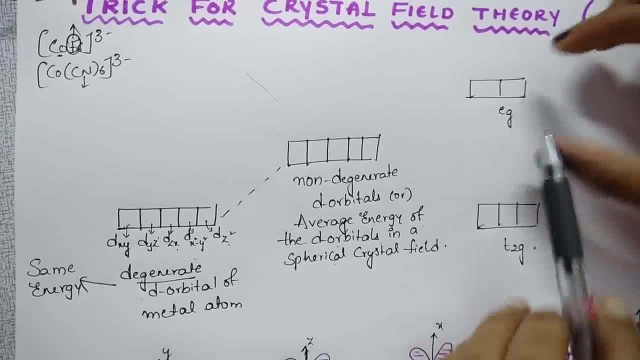 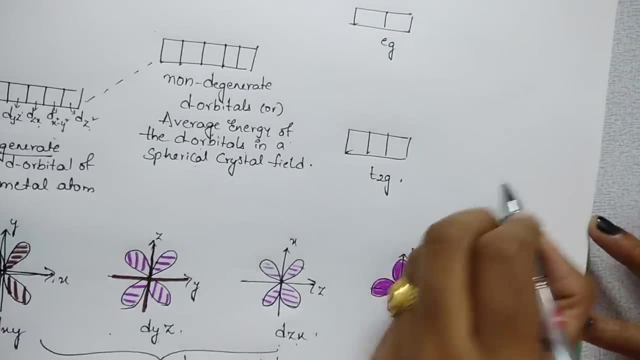 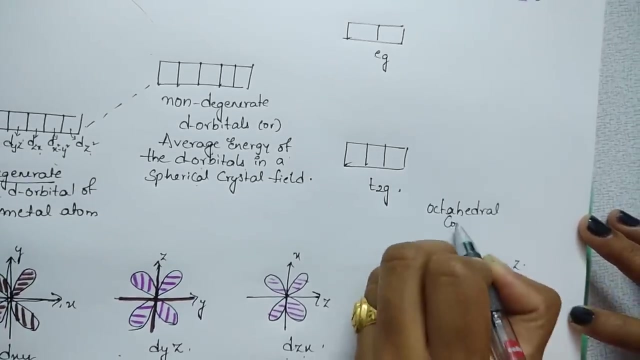 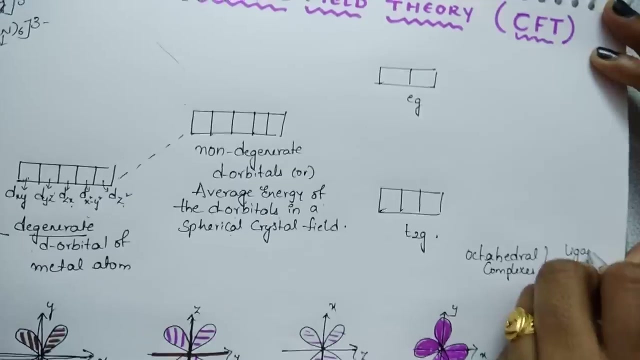 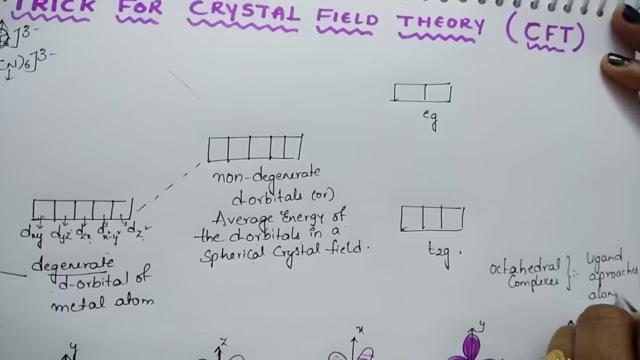 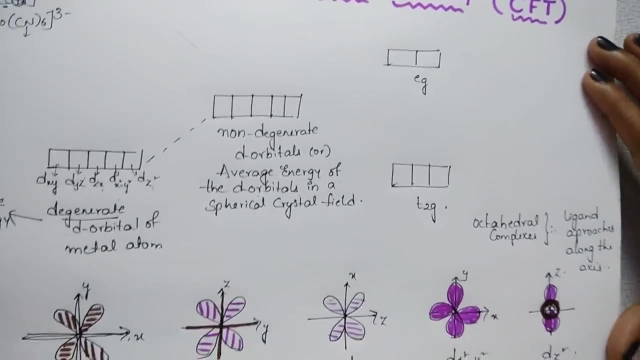 and see here, if you observe carefully, this EG set lobes are present along the axis we already discussed. and in the case of octahedral complexes, octahedral complexes ligand approaches along the axis and whose lobes are along the axis students, EG, orbital lobes are along the axis. 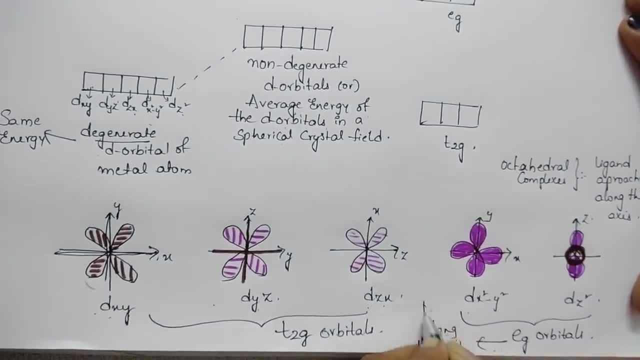 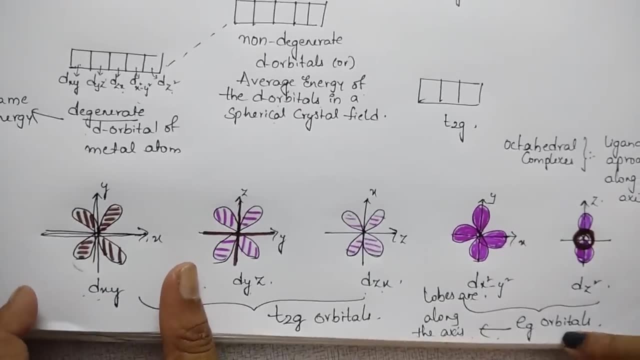 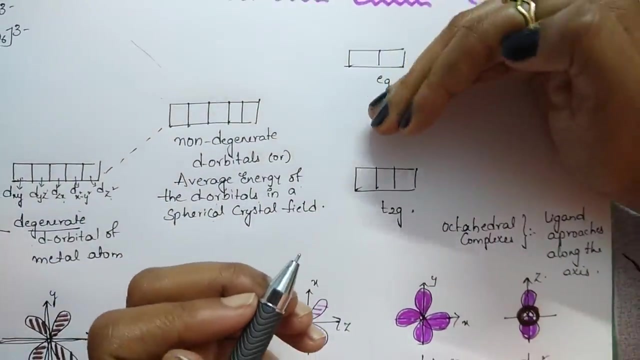 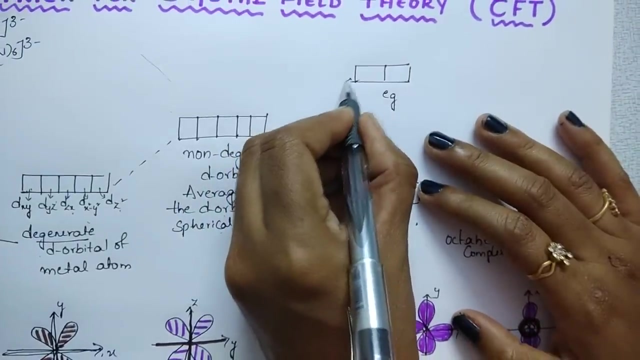 lobes are along the axis. whenever EG lobes are along the axis, then in the case of octahedral, what is happening? ligand is approaching along the axis and EG orbital lobes are also along the axis. so these 2EG orbitals, energy is raised and, if you observe, 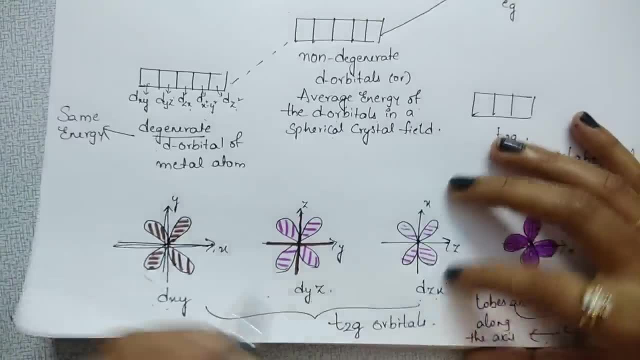 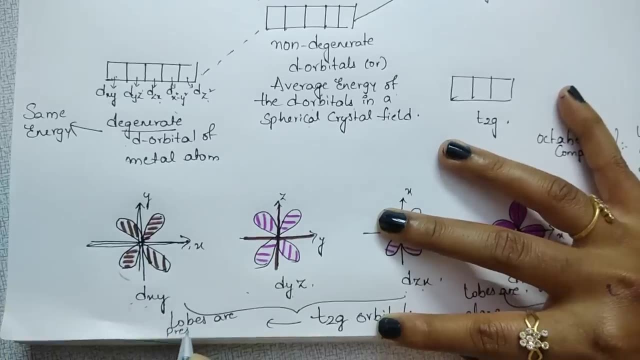 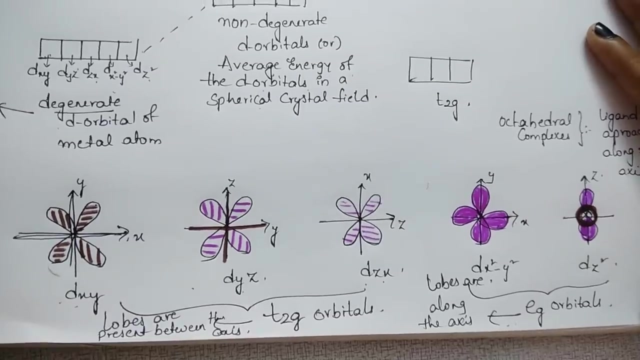 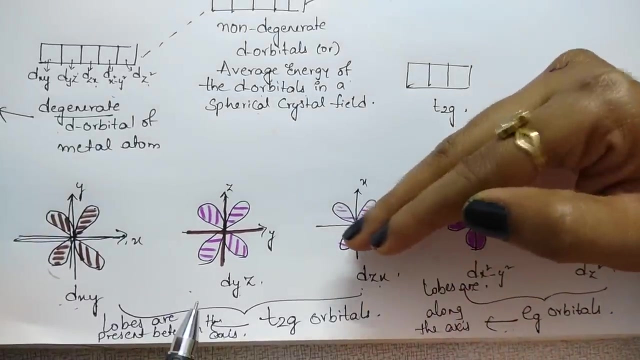 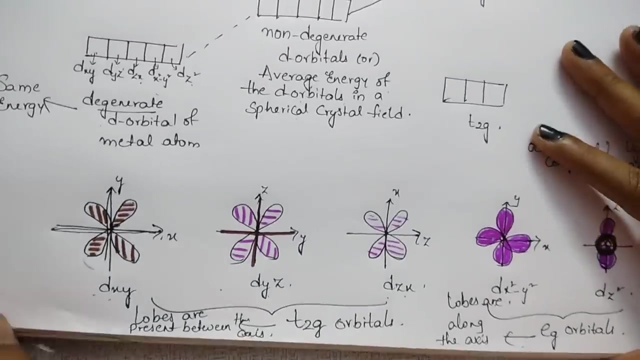 here. T2G orbital lobes are present between the axis. T2G orbital lobes are present between the see. T2G lobes are present between the axis, so ligand is approaching along the axis, not in between the axis in the case of octahedral complexes, then. so T2G orbitals experiences. 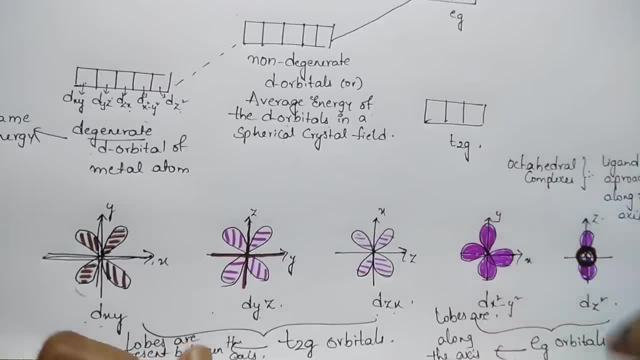 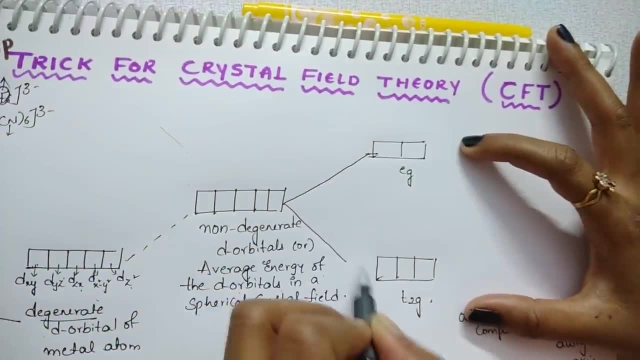 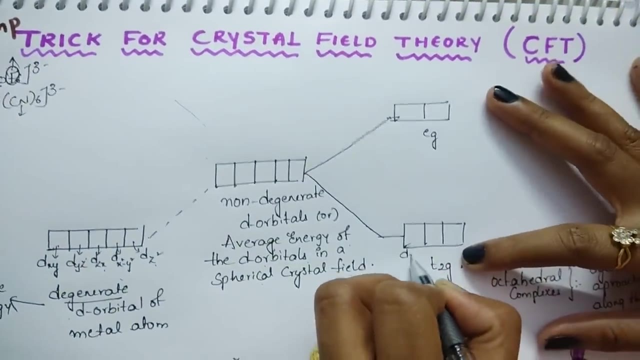 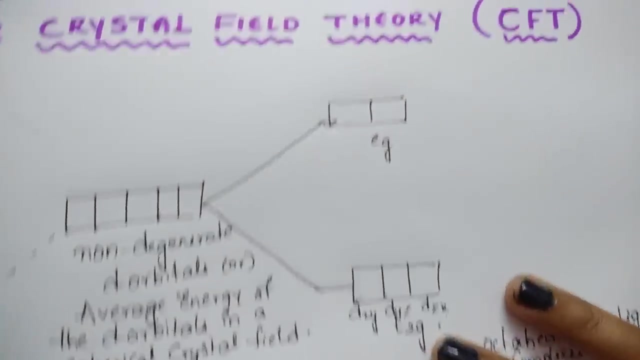 very less repulsive forces, so they goes to the. their energy decreases. see here the energy gets lowered. T2G orbital. what are those three T2G orbital students? dxy, dx, dx, dxy, dyz and dzx? these are T2G orbitals. and what are EG orbital students? EG are dx square. 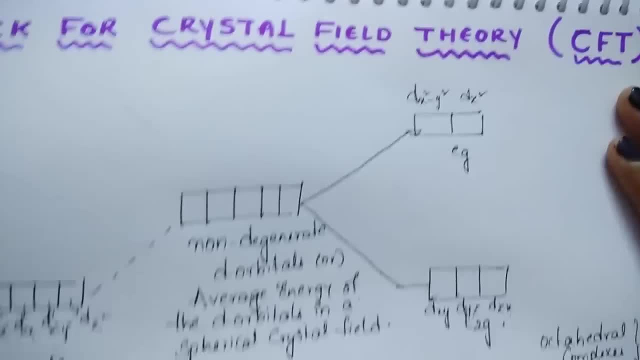 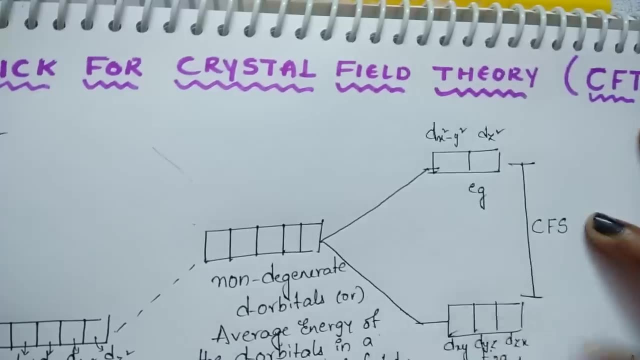 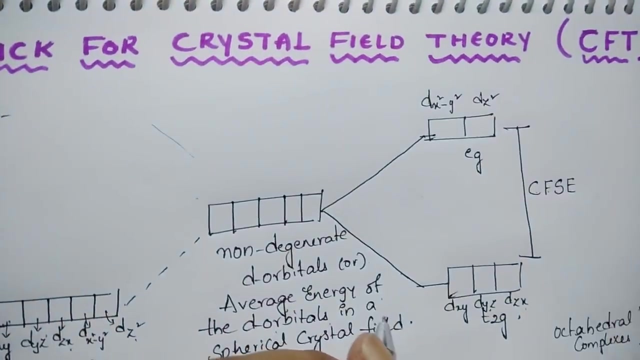 minus y square and dz square are EG orbitals. if you see this splitting, we call it as crystal field splitting or we call it as crystal field stabilization energy or splitting energy. what do you mean by this crystal field splitting energy, this difference of energy? 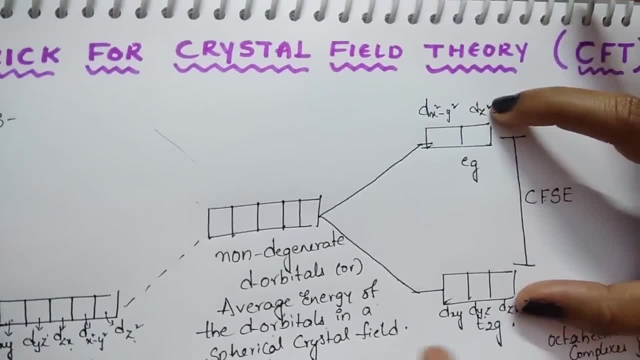 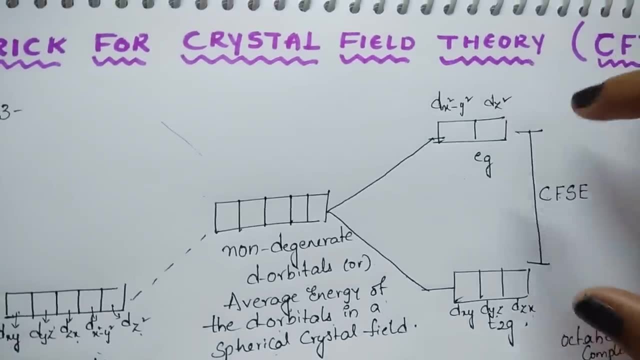 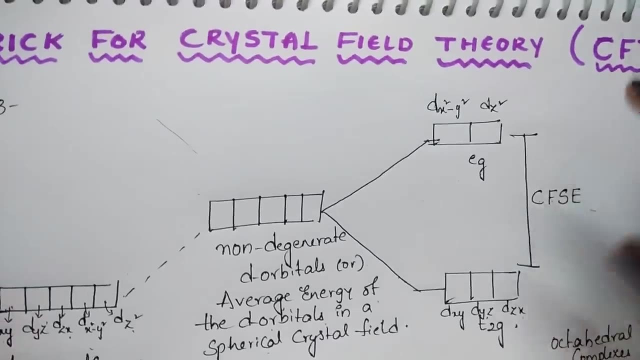 between these two set of degenerate orbitals. as a result of crystal field splitting energy. we call it as. as a result of crystal field splitting, we call it as crystal field splitting energy, or which is also known as crystal field stabilization energy. the energy difference. 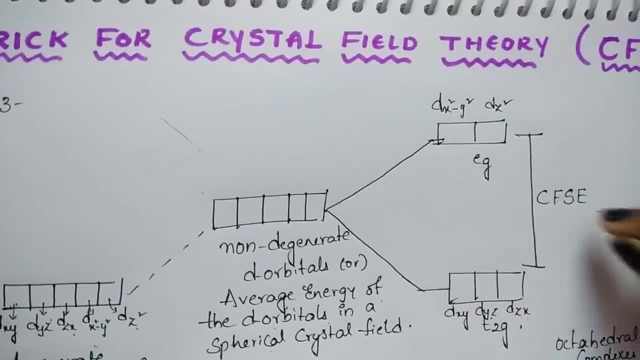 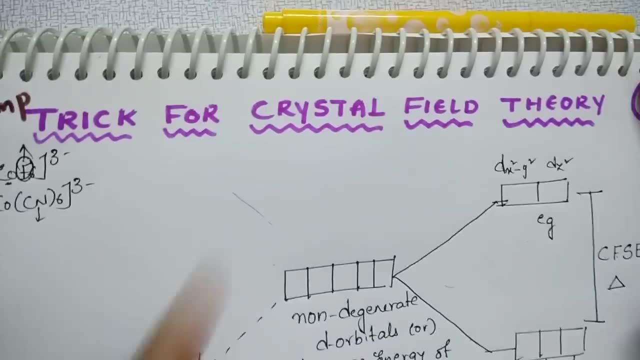 between these two. we call it as what? crystal field stabilization energy, which is represented by delta, and we are discussing in the further octahedral complexes. so these are the two octahedral complexes for what we are discussing here. how many legands are there, students? 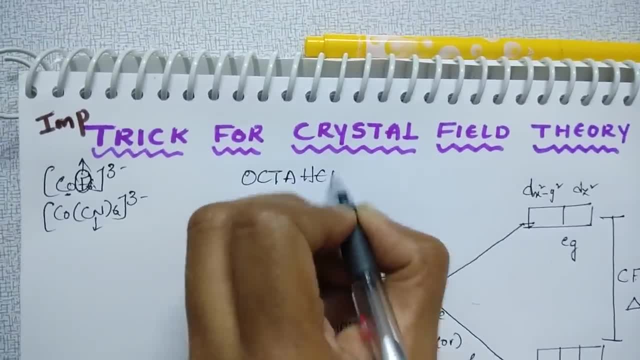 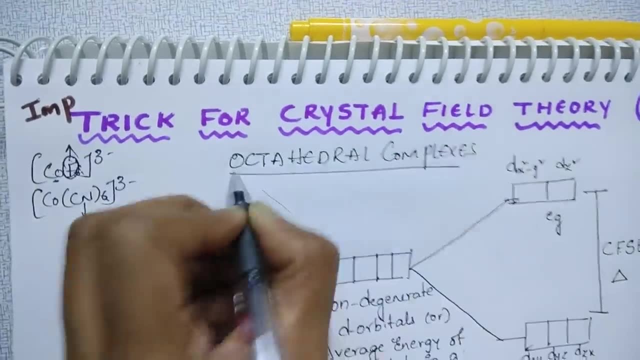 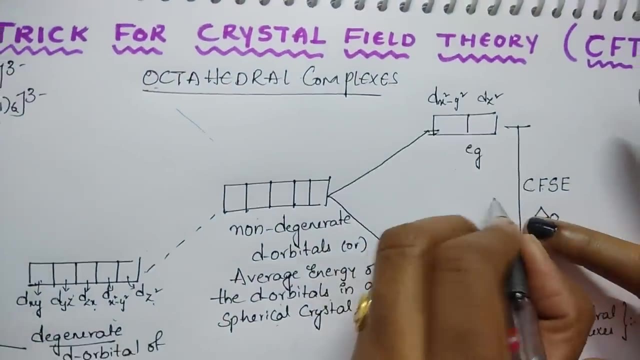 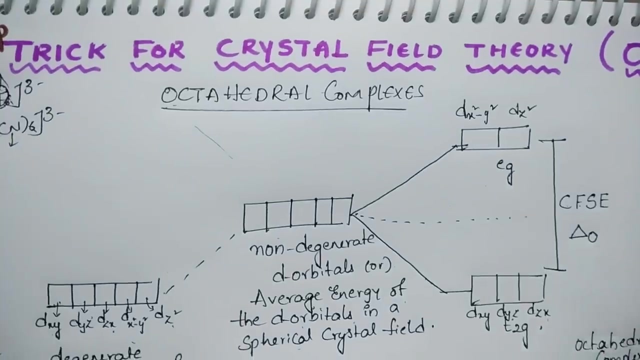 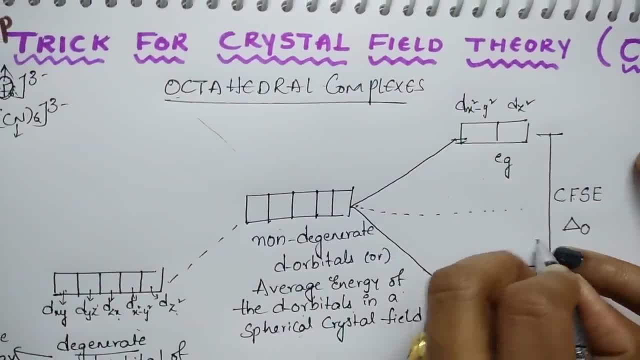 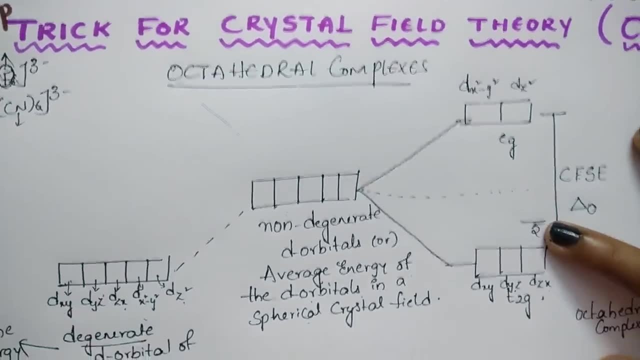 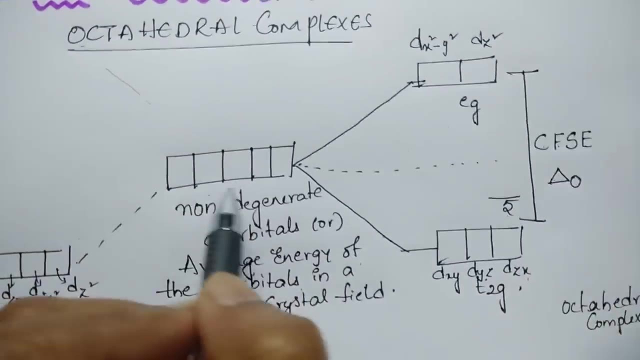 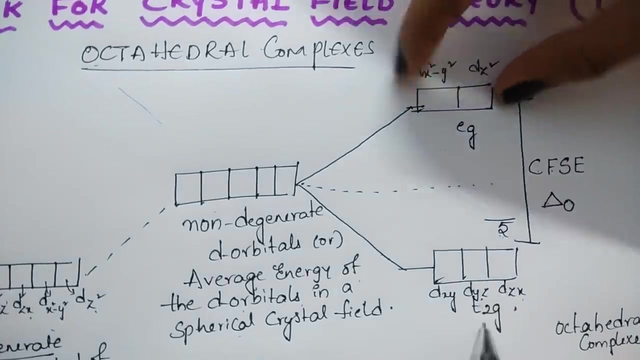 students. we are going to also get rid of this T2G as much as we can in the future- and some other principles give the completeness to this T2G- and we are going to search the recuperation of these almost increasing chimneys. so now let's look at the complicity of 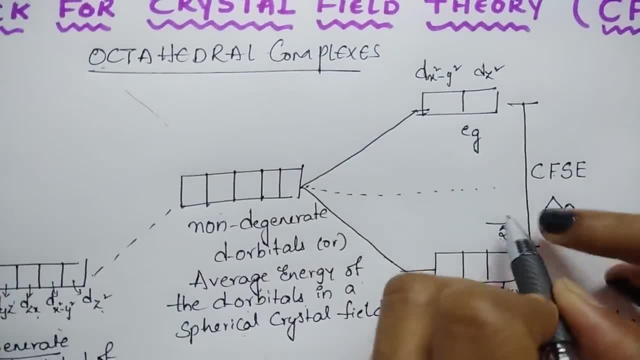 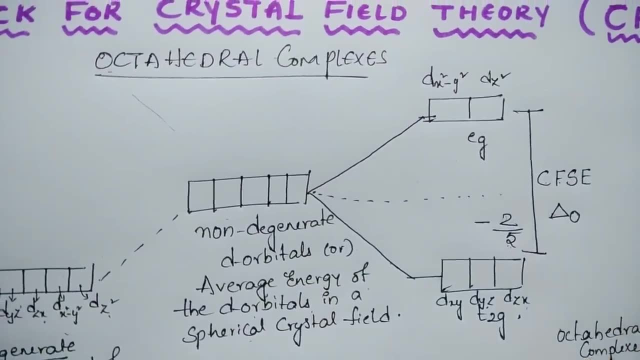 these elements one by one. So when we consider the ion deformation and its ribod GRA- you may have named these as ther alimentos in here- general electron activity. so among how many? among 2 and T2G orbitals, energy are decreased. so minus 2 by 5, and this is for. 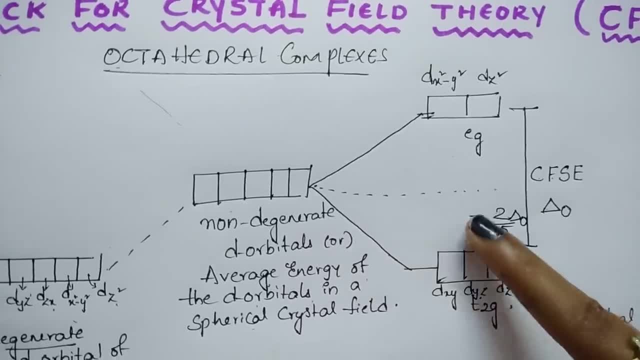 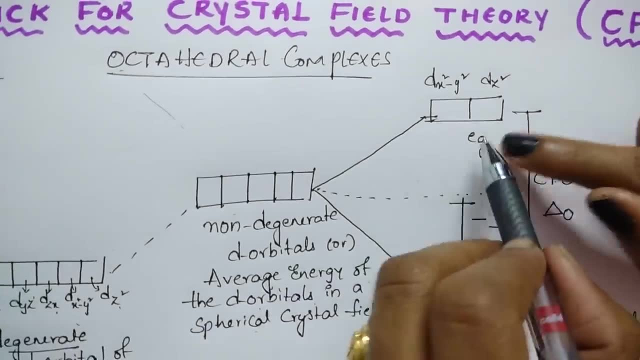 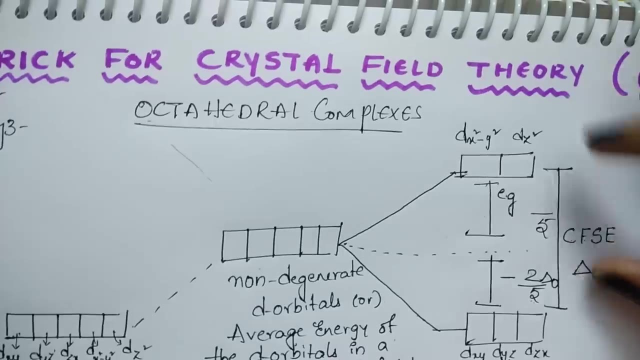 octahedral complexes, CFSE. that's why minus 2 by 5 delta naught for T2G. this is for T2G and, in the case of EG, for total 5 d orbitals among 3 d orbitals. this EG orbitals energy is. 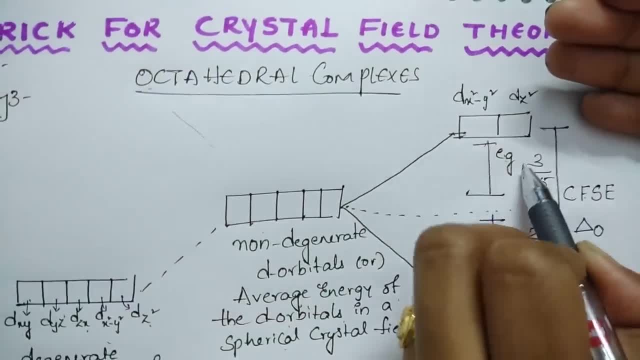 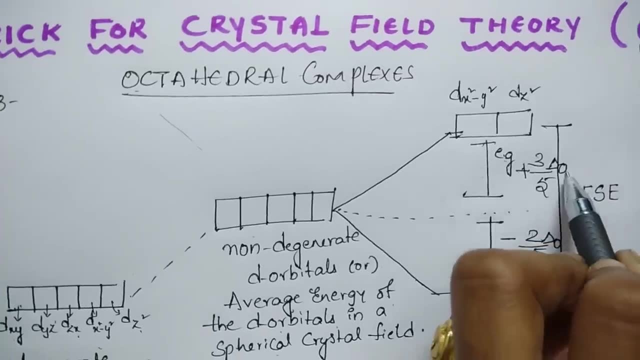 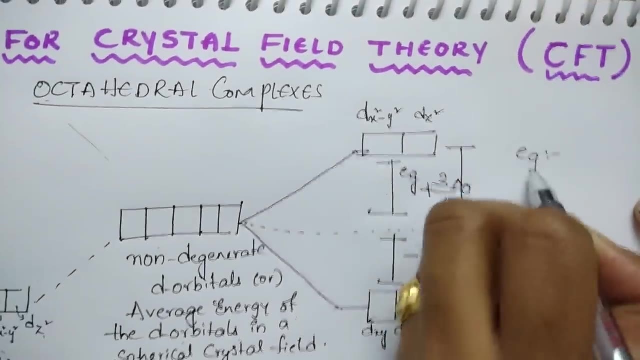 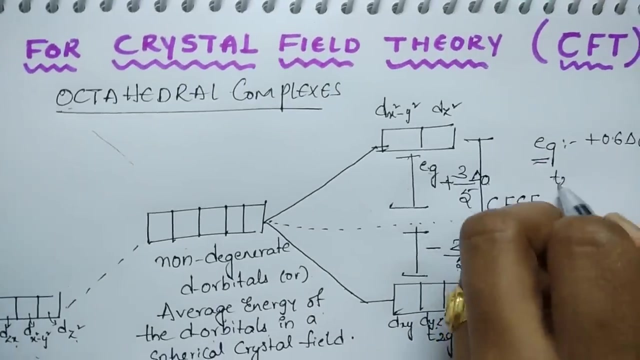 increased means. 3, its energy is raised, positive sign and delta naught for means. delta naught not indicates, O indicates it is for octahedral complexes. so EG: what is the EG? CFSE value, students, what is the EG value? 3 by 5 means plus 0.6 delta naught and T2G: what is? 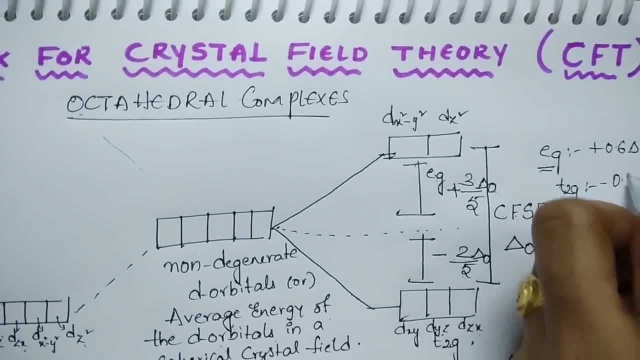 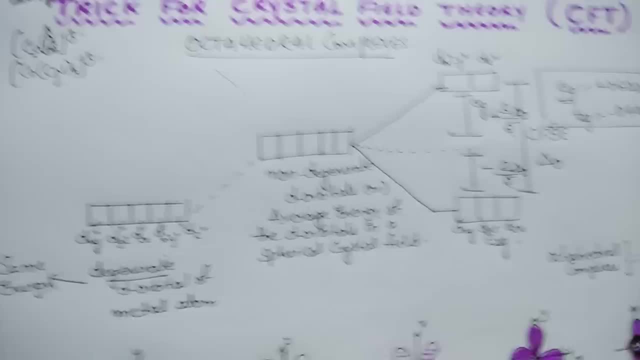 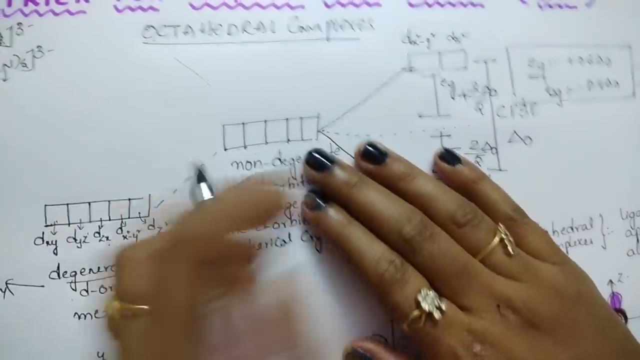 the value for octahedral complex minus 0.4 delta. naught. see here first what you do in your exam: just draw 5 d orbitals. this 5 d orbitals energy is raised first. draw 5 d orbitals. energy is raised. you mention it. 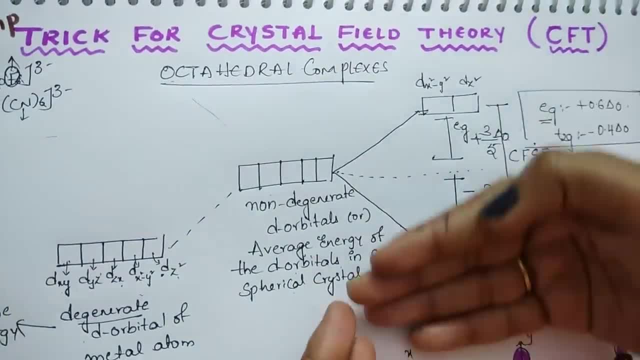 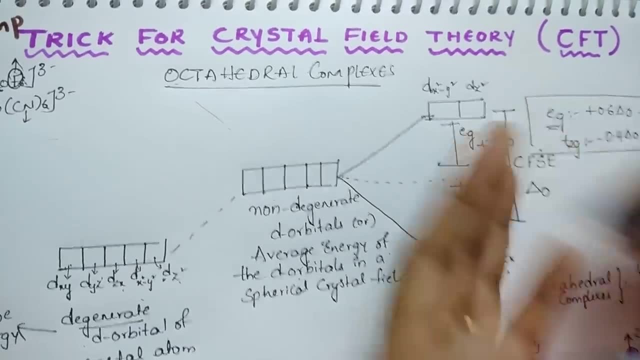 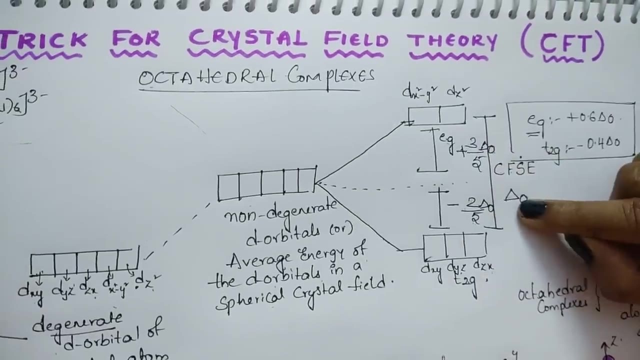 as average energy of d orbitals. when ligand approaches, then d orbitals splits up into two sets. one is called as T2G set, another one is called as EG set, and the total energy difference between these splitting we call it as delta naught and the energy difference is delta naught. 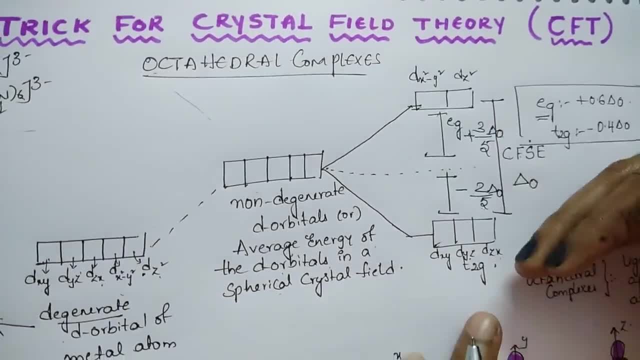 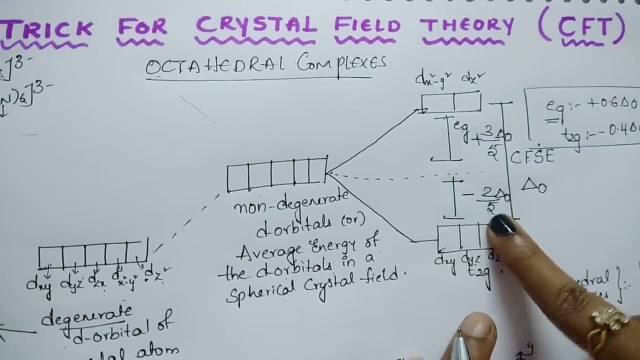 and EG and T2G, T2G. how much students? total 5 d orbitals are there among 2 d orbitals. its energy is also minus 2 by 5 and it is energy is increased among 3. that is why it is plus 3 by 5 delta. 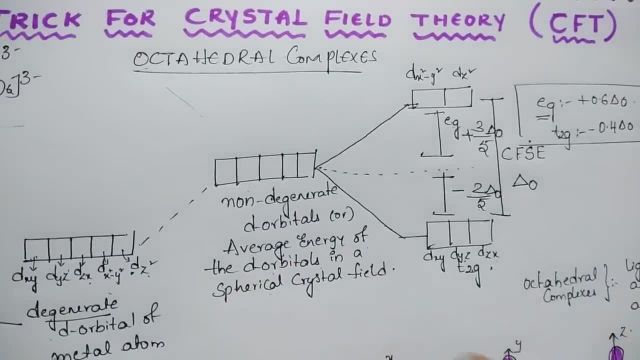 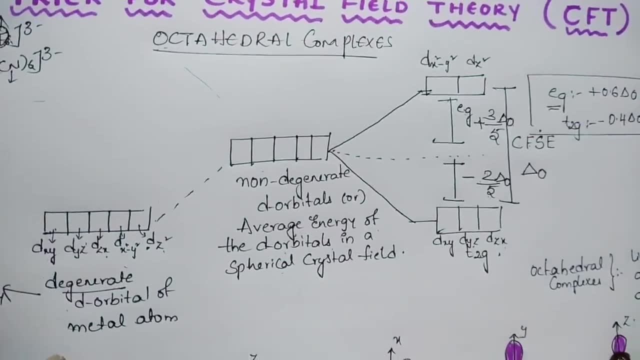 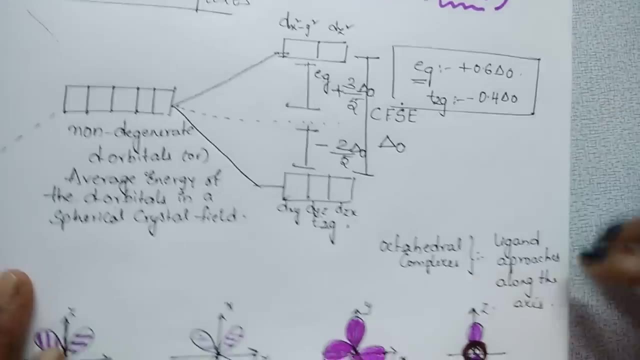 naught, and this is for SFIC. beautiful theory for octahedral complexes. in the case of Tietra Hedl complexes also, the same thing will happen, but let us see the diagram for that. just the reverse of this. because in the case of tetrahedral complexes what happened, see in the case of 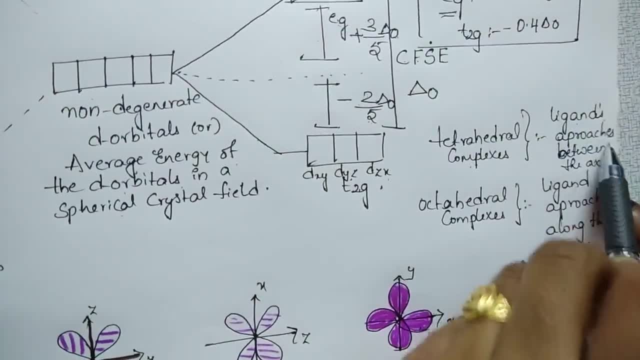 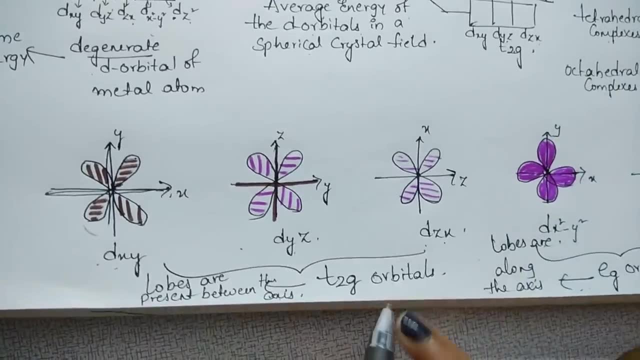 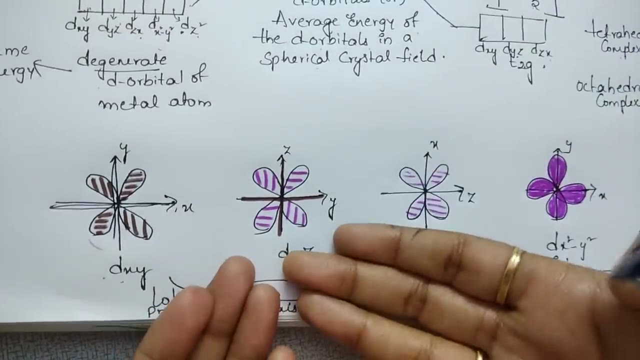 of tetrahedral complexes. ligands approaches between the axis. Whenever ligands approaches between the axis whose lobes are between the axis. T2G orbital lobes are between the axis, So which orbitals goes to the higher state? T2G orbitals. This here you should write T2G. 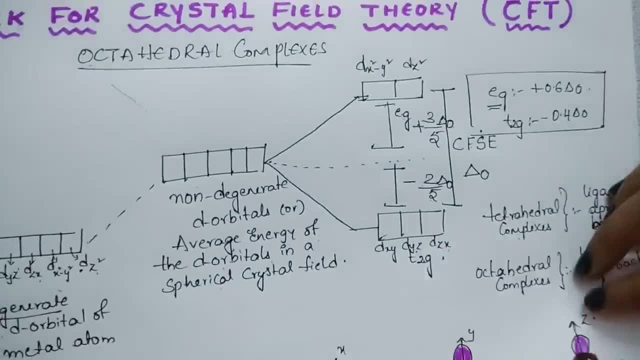 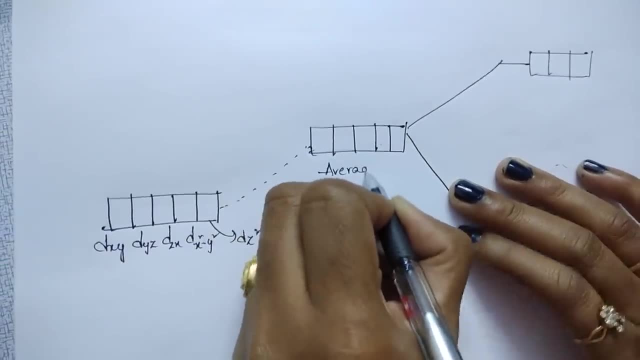 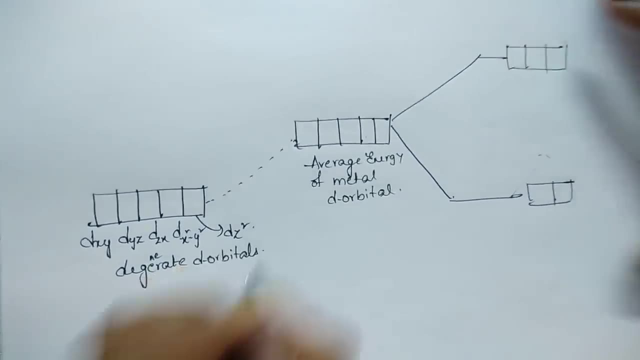 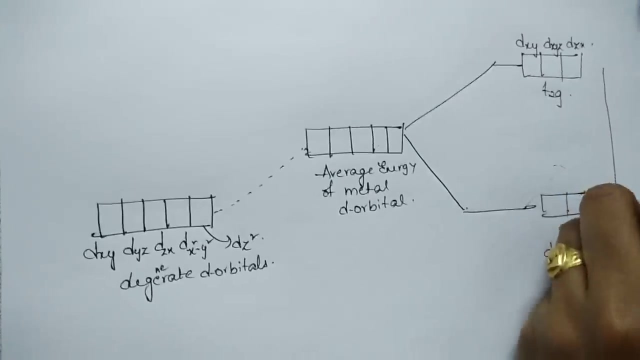 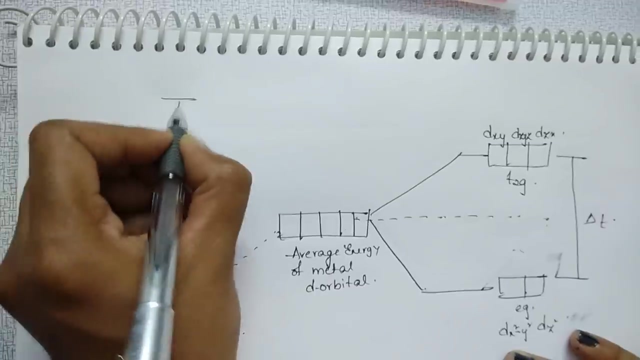 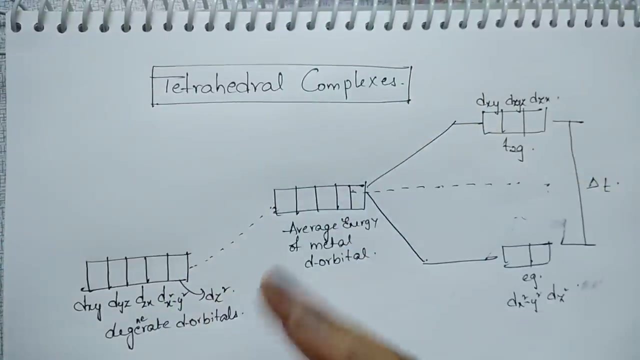 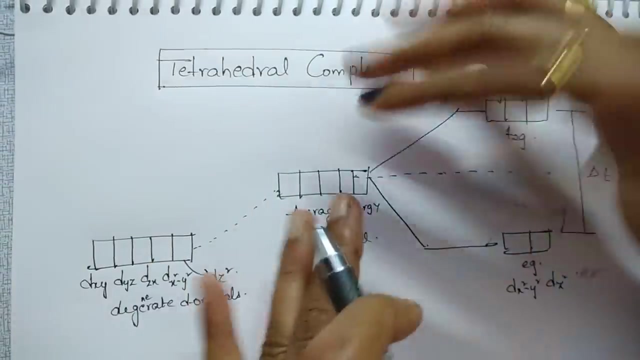 here you should write EG. Well, see the diagram. See, in the case of tetrahedral complexes, what you do is just take the D orbitals, 5D orbitals. When the ligand approaches the 5D orbitals loss the degeneracy and 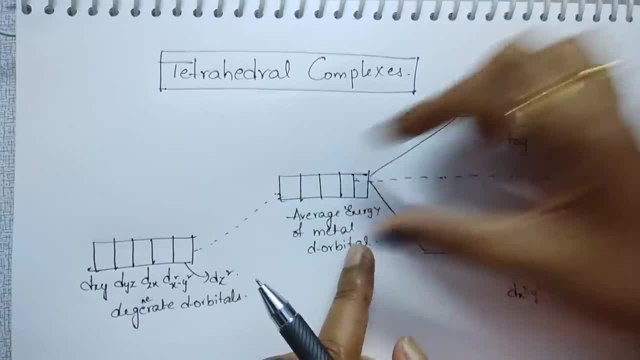 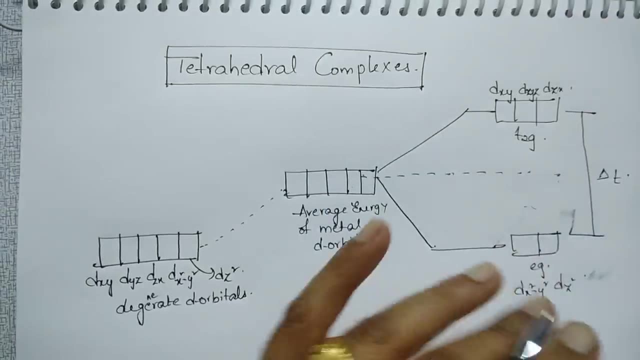 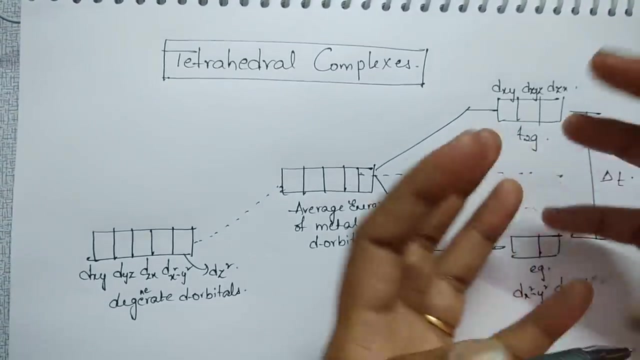 comes to the excited state and these 5D orbitals splits up into two sets, In this case of tetrahedral. what happens is the ligand approaches between the axis. T2G orbital lobes are between the axis, So these T2G orbitals experiences more repulsive forces. 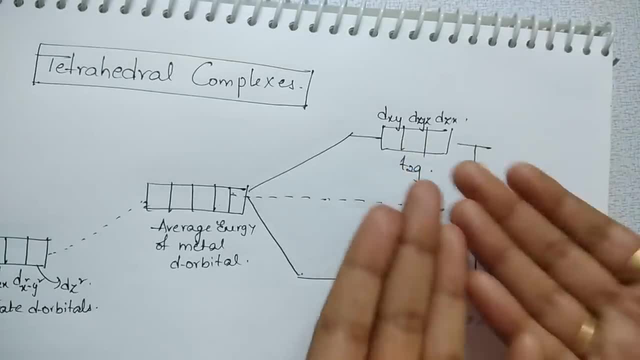 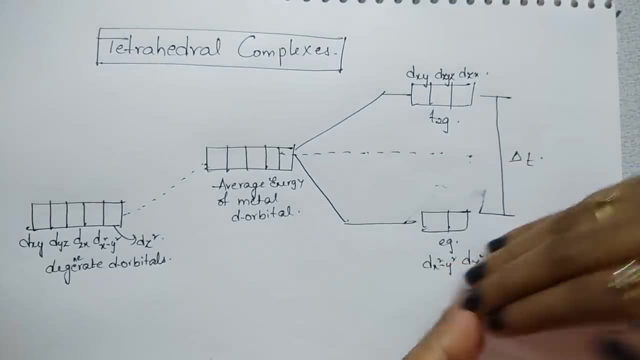 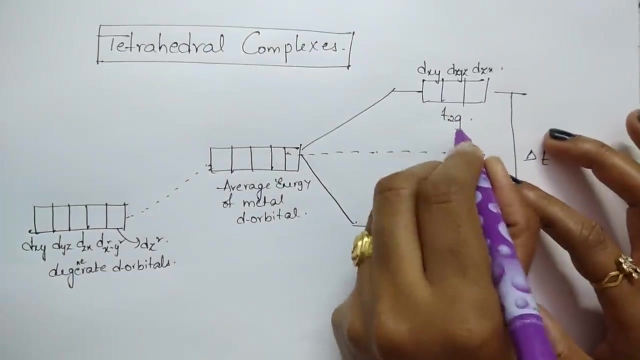 and goes to the excited state, and this is the excited state of T2G orbitals And EG orbital- experiences less repulsive forces, they comes down And the main thing in the case of tetrahedral is, according to the spectroscopy, you should not represent a Garrett symbol. for this, Don't write a G, okay, While you are writing. 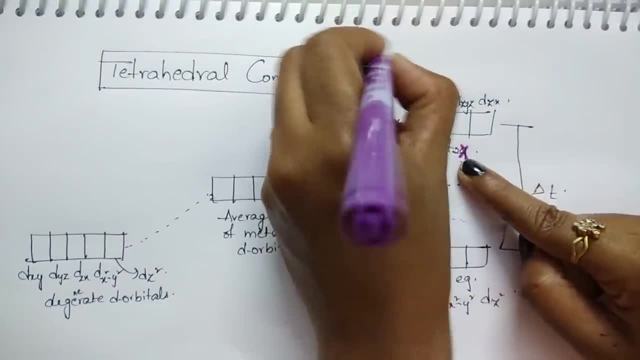 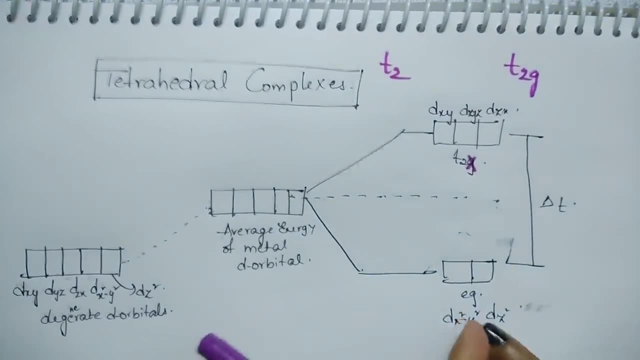 your exam, mention only T2 for tetrahedral And in the case of octahedral, T2G right. And in the case of tetrahedral, you should not write a G. So you should not write a G. So you should not. 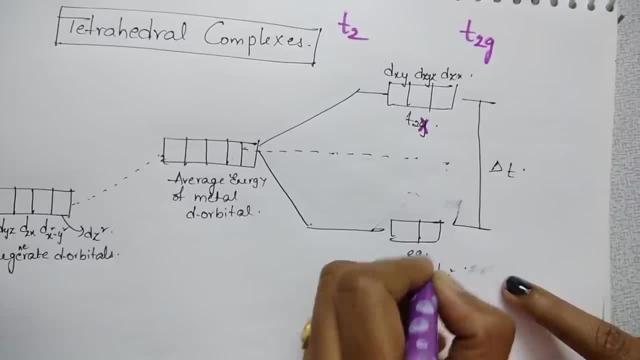 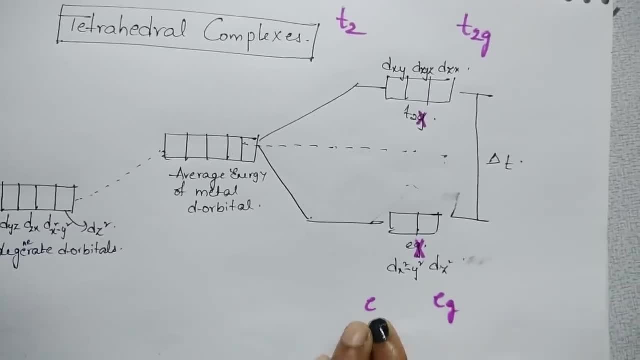 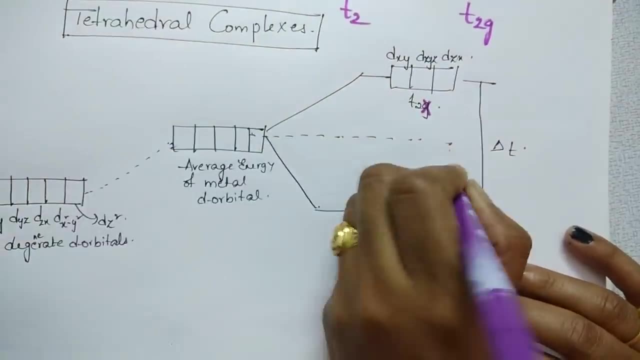 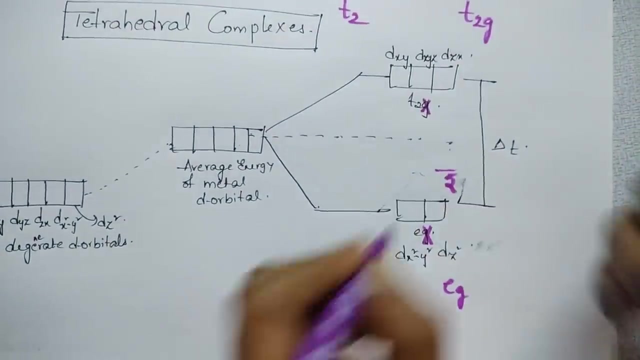 you can represent EG Only: E in the case of tetrahedral and EG in the case of octahedral. fine, And here, out of total 5 D orbitals among 3 orbitals, EG means E orbitals are decreased.